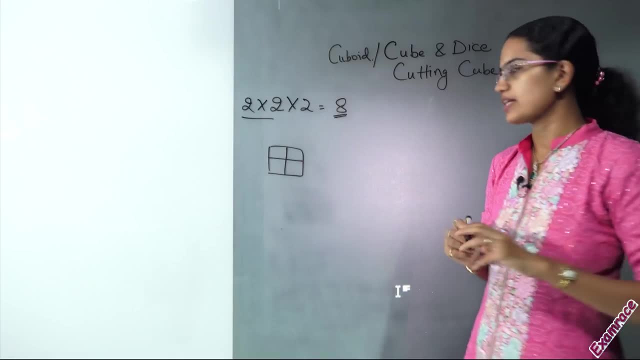 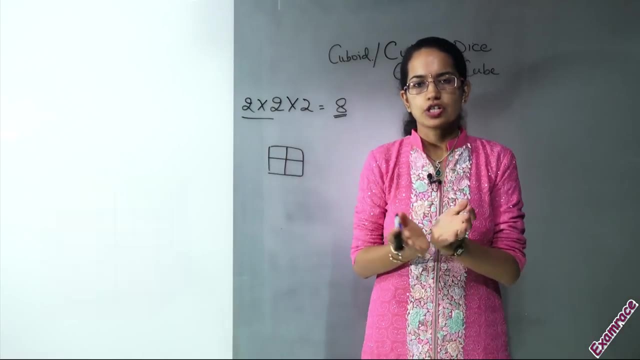 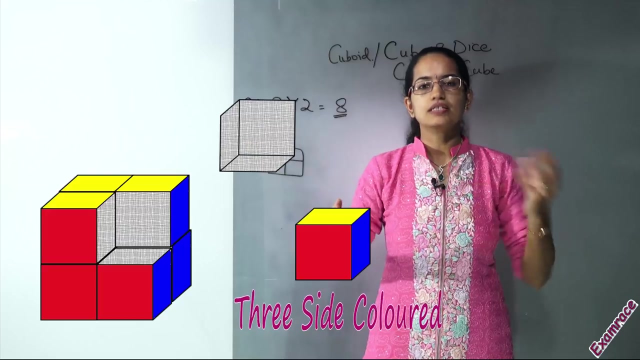 which would have three sides as painted, would be always eight. Now in this case, you can clearly imagine it. I have a cube here. I have cut it into eight pieces, So each of the piece that remains would have three sides as painted. 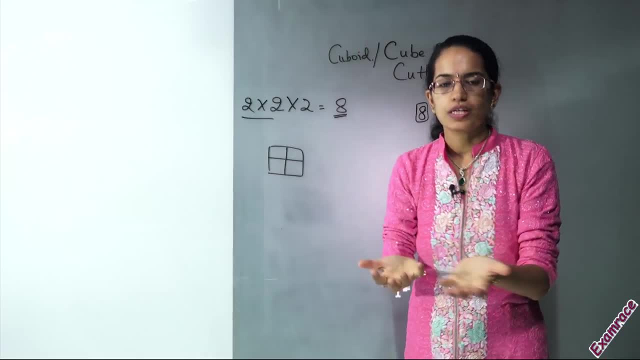 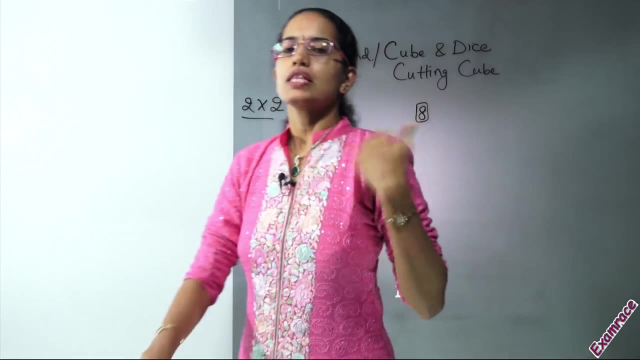 So since there are total eight cubes, and all of the eight would be three sides as painted, there would be no cube with one side, zero side or two side that would be painted. Now consider another case where I have a 3x3x3 cube. 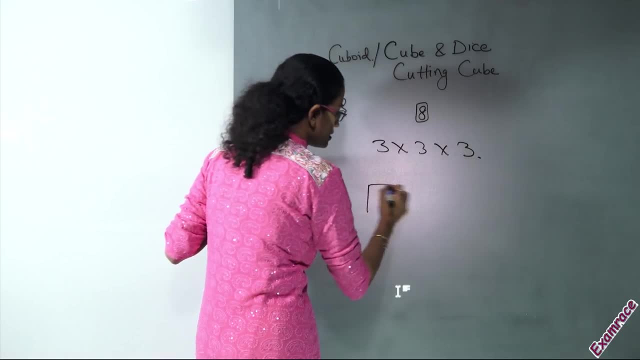 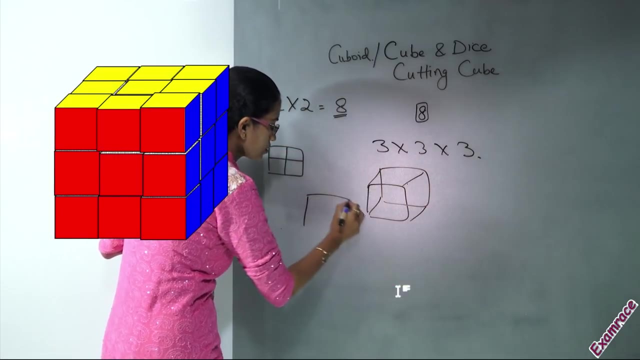 Now, in this 3x3x3, what would happen is, let's say, I have a cube here and in this cube let's pick out one surface out of here and what I'm doing is I'm cutting it into three 3x3. 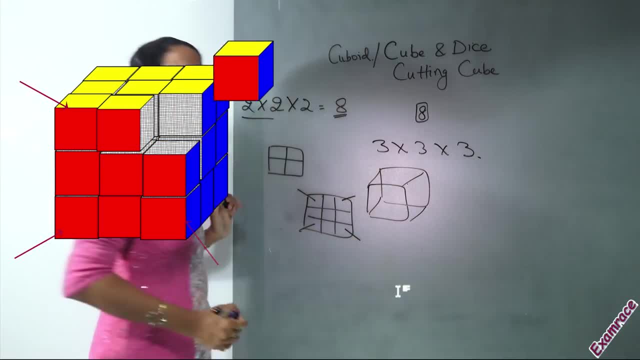 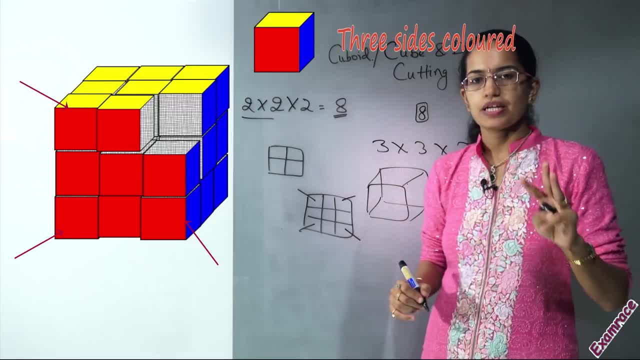 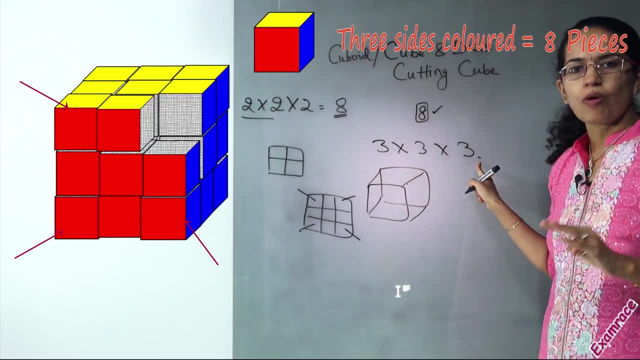 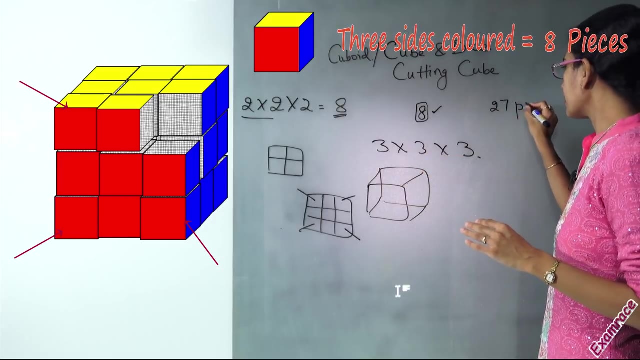 Where you have cubes. you would have three sides as painted. How many pieces would be there? There would be eight pieces, as always. Now, how many total number of pieces would be formed in a 3x3x3?? So in a 3x3x3, you would have 27 pieces that would be cut up. 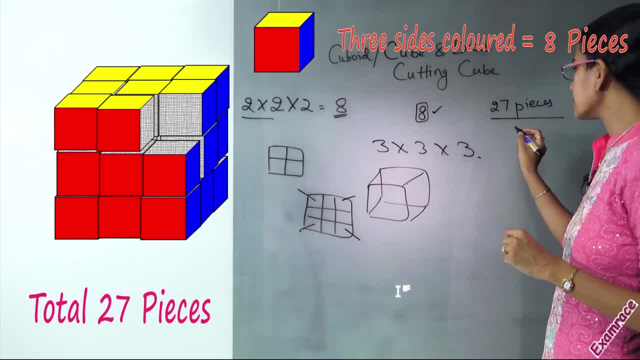 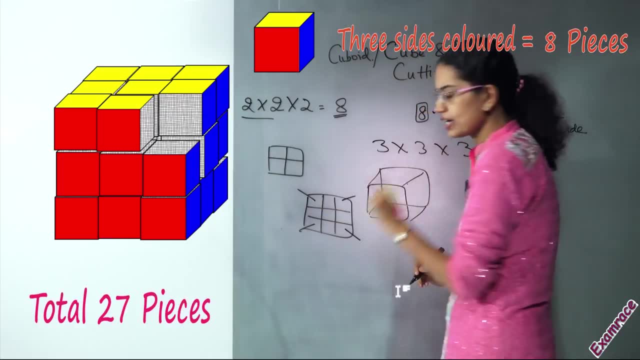 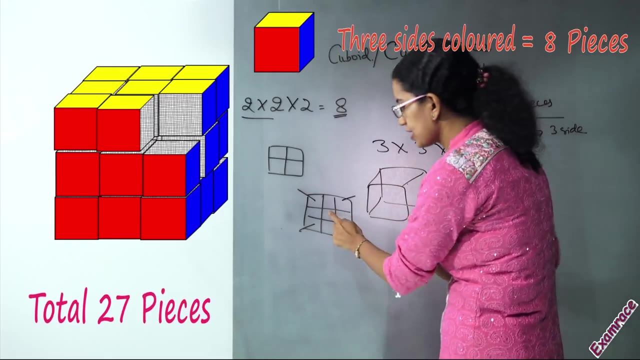 Now these 27 pieces. of these 27 pieces, you would have eight which have three sides as painted. Now these are the ones which have three sides as painted. The easiest thing under a 3x3 cube would be the center one. 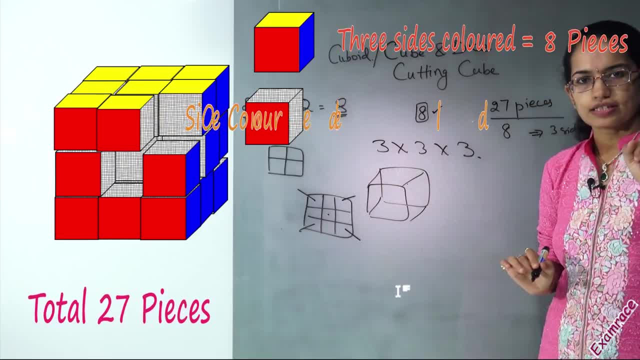 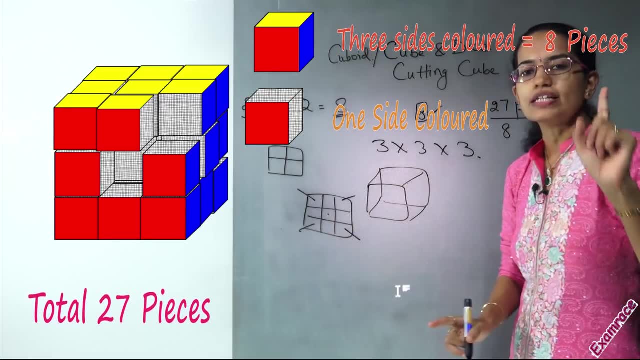 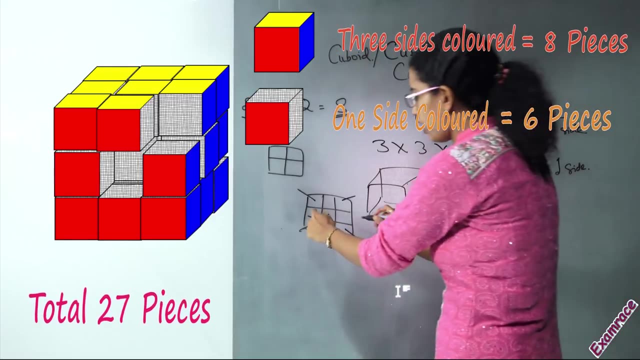 So this piece would have only one side as painted. And how many faces for a cube? Six faces. So how many would be the piece with one side as colored? So there would be six pieces which have one side as colored, Again the outer ones. you would have two sides as colored. 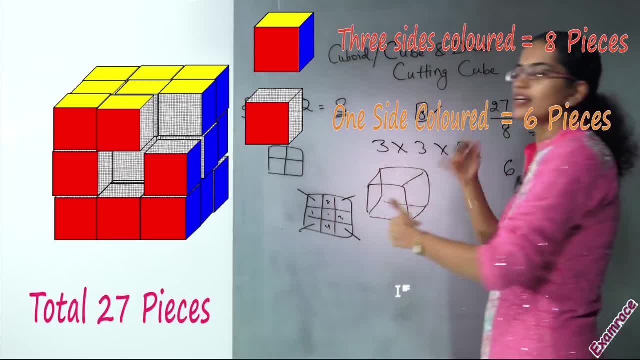 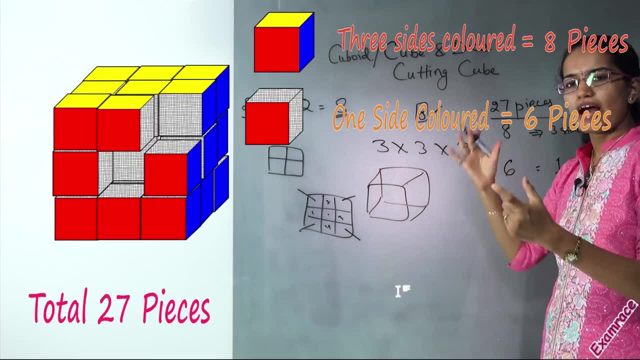 So you would have one, two, three and four this side, Four on the back side, So four in the front, four in the back And then two and two here. So you would have four, four, eight and four, twelve. 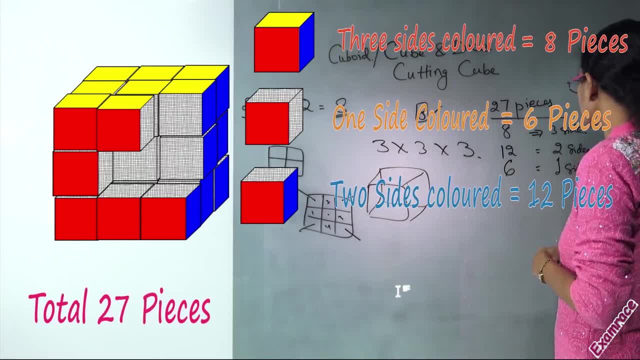 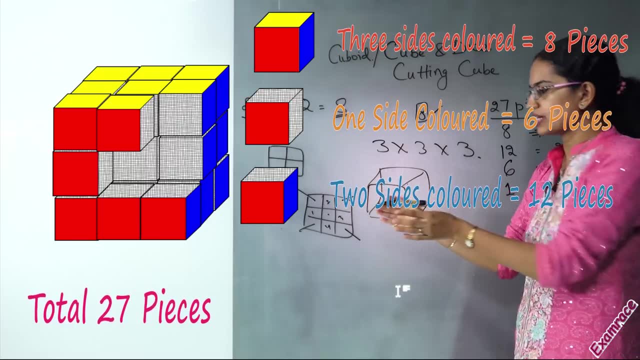 So you would have twelve pieces, which would have two sides as painted, And finally, when I add this, this comes to 26.. I have one more piece that remains within the center, So let's consider this cube. I remove the first layer. 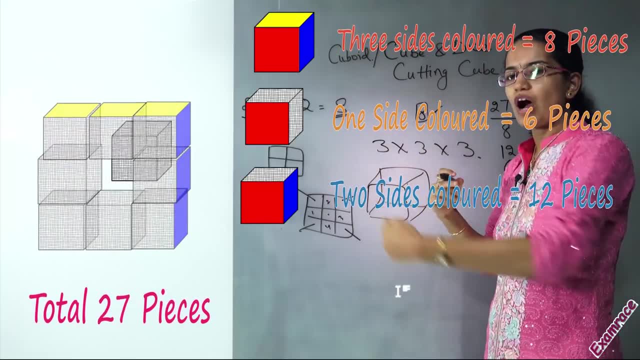 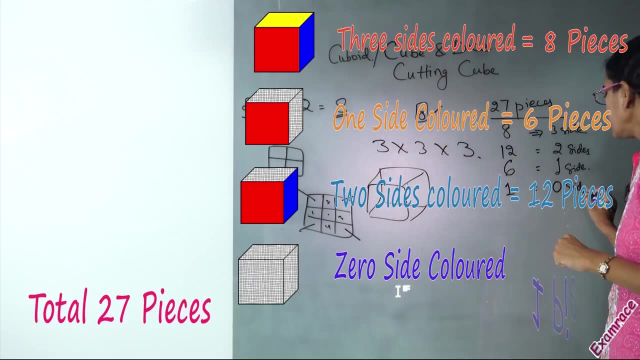 I remove the last layer Of the middle layer. I remove all the outer ones. So how many cubes remain in between Is one, And therefore you would have one cube which would have zero side as painted. So that's how we solve a 3x3x3.. 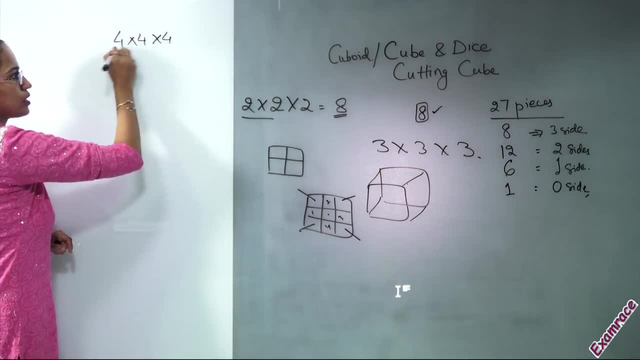 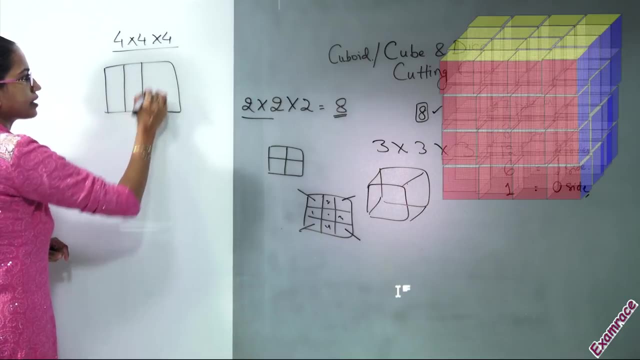 Now let's come on to a 4x4x4 cube, Interestingly the same cube that we have here. I am taking just one surface of it, So what I am trying to do is I am trying to cut it into 16 pieces. 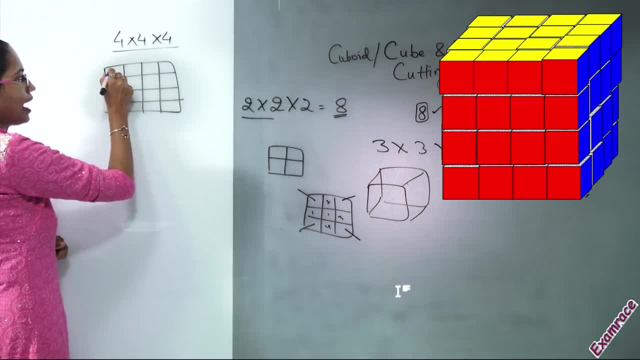 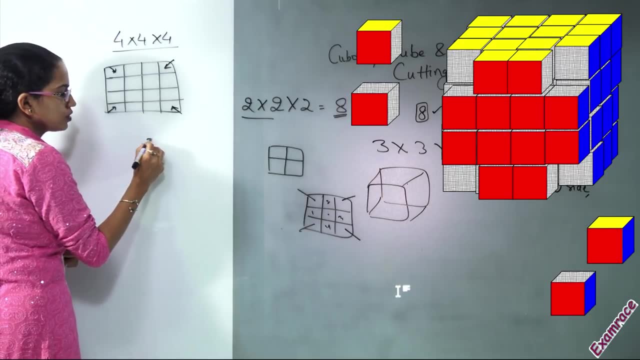 So that's the only surface I am visualizing as of now. So I have one. So the corner ones that would be gone in three sides painted. So again as we know, three sides painted. how many cubes would be there. 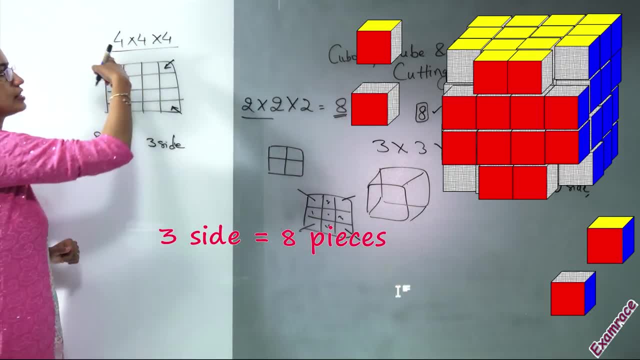 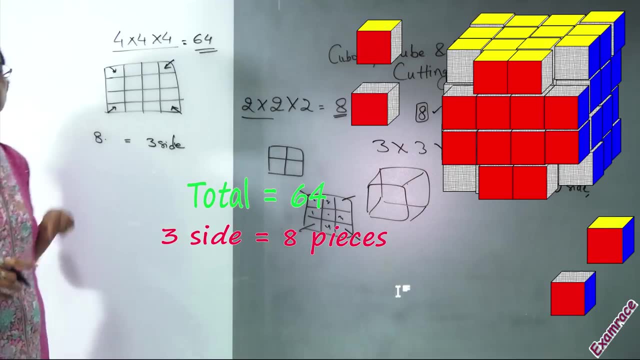 There would be eight cubes And 4x4x4, that's 4x4, 16x4, 64 would be the total number of cubes. Now what I do is I find out the cubes which have two sides painted. 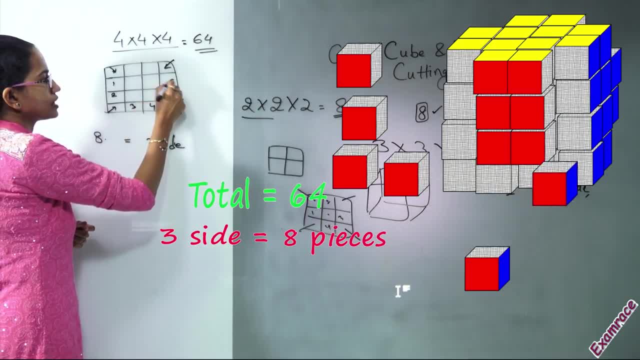 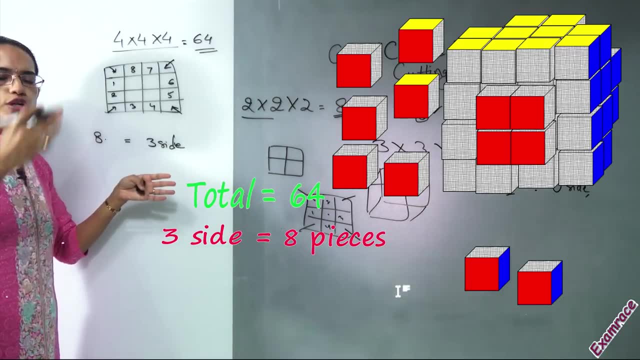 So one, two, three, four, five, six, seven and eight, Eight in the front, eight towards the back surface. Then you would have a total of four here and four here on the either side. So 8 plus 8, 16.. 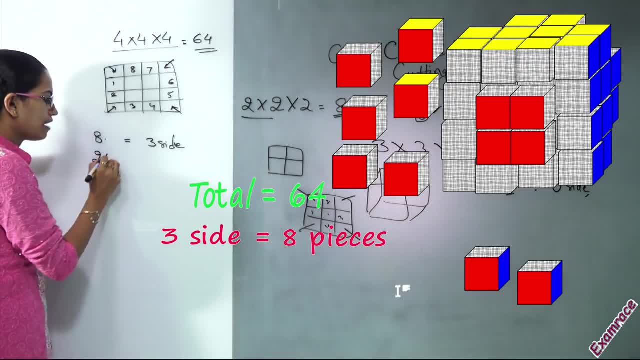 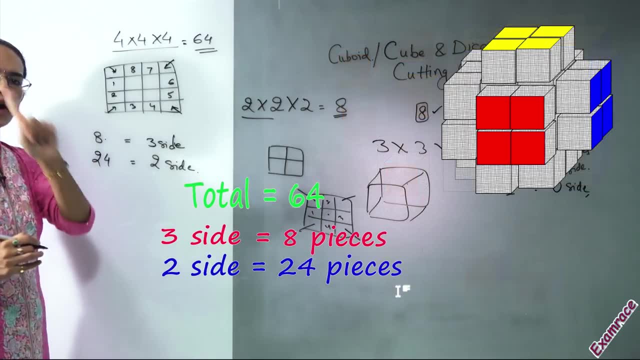 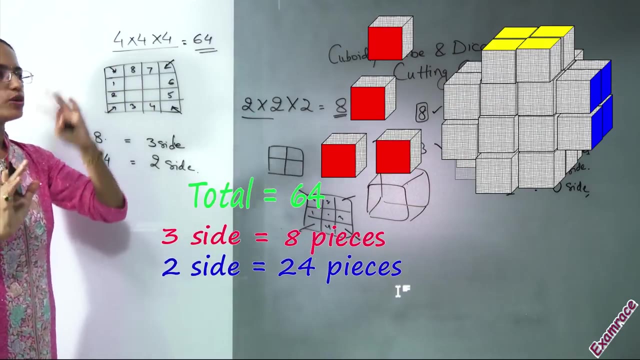 16 plus 8, 24.. So you would have 24 pieces which have two sides colored. Now, how many pieces would have one side colored? You have four in one face, How many faces a cube has? As we know, in the starting we talked about the six faces of the cube. 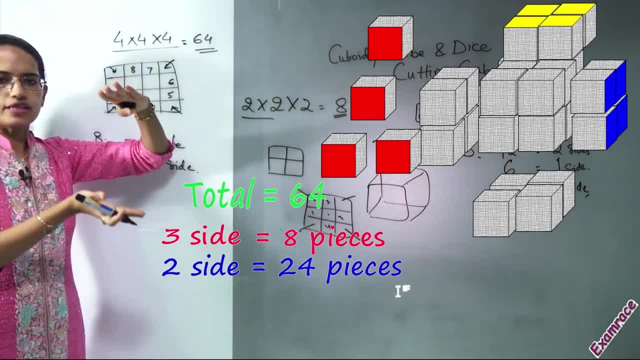 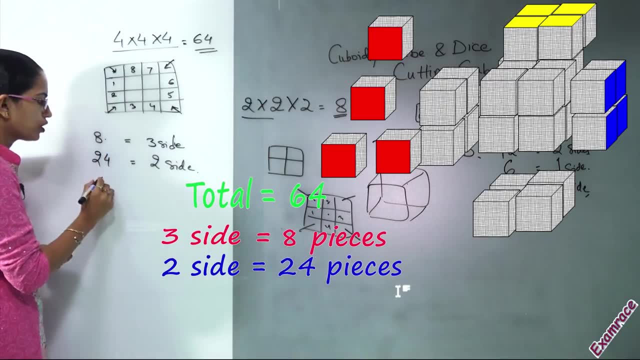 The four on the four sides are top and the bottom, So on each of the face you would have how many faces which are one side colored. That would be four, So it would be 4x6, that's again 24.. 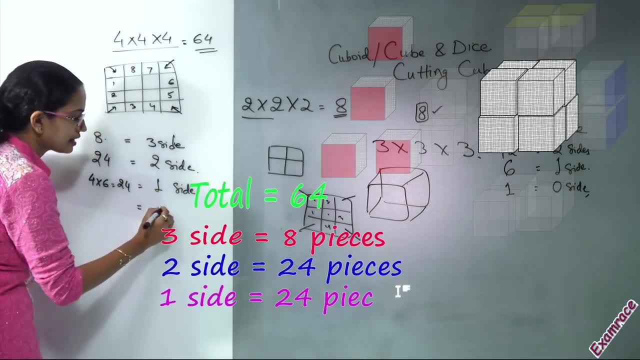 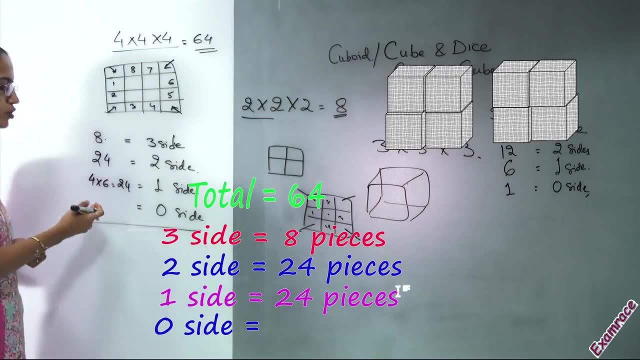 And those would be one side colored. So how many would be zero side colored? Now, one of the simple ways is I add all of those and subtract that from 64. So I get the value. Or what I can do is, since it's a 4x4 cube, 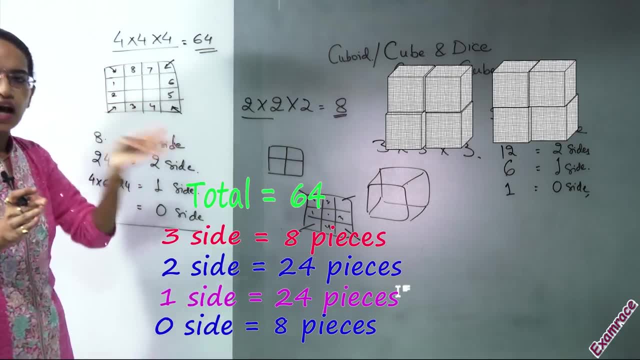 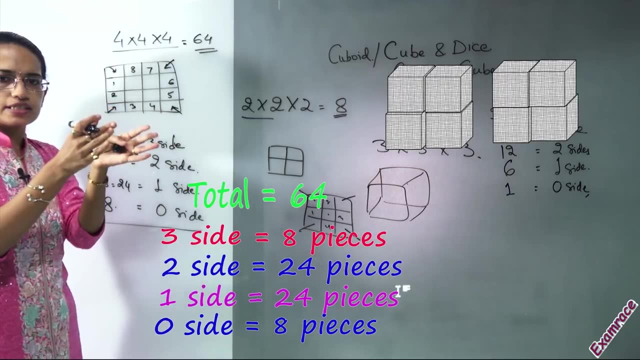 So I remove the outer. the first layer, that's this one, The last layer, that's the other one, And in between I have two layers that remain, So 16 and 16 pieces in the middle. I remove all the outer pieces. 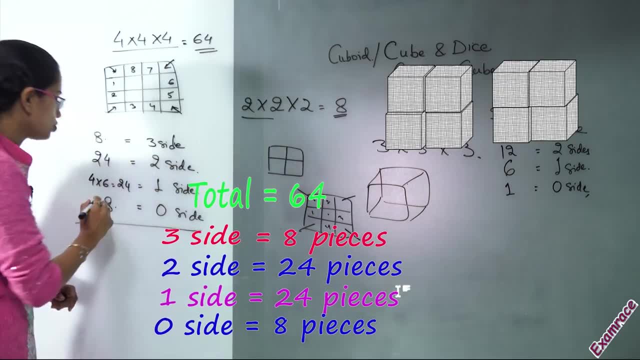 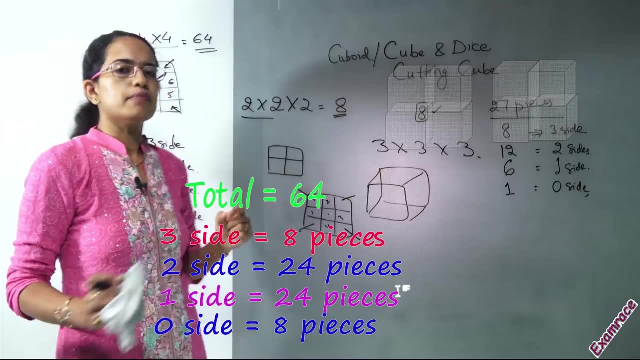 So how many pieces remain in between are 8.. So those 8 form the number of cubes which have zero sides as painted. Now, that was a simple method to understand, and this we can continue further Till 5x5, 6x6 and so on. 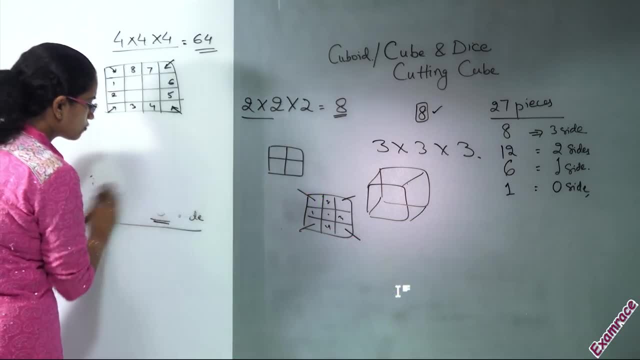 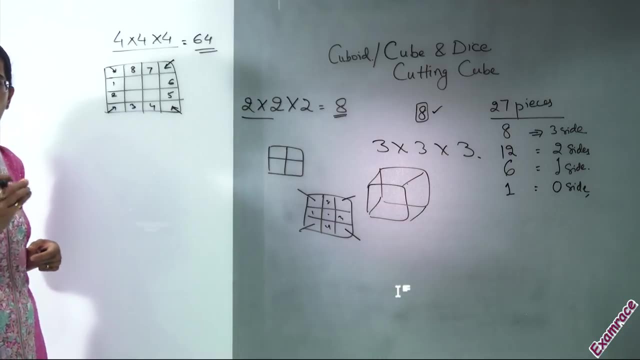 Now, what is a method or a kind of quick trick to remember the number of cubes or number of sides that we can derive? So I have a simple formula for you For three sides. in case of cube, as I said, it's simplest to remember. 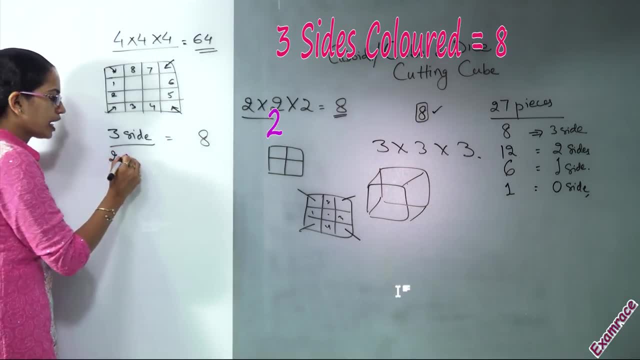 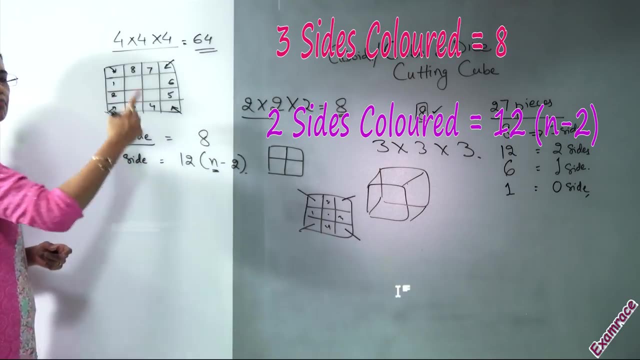 You just need to put 8.. For two sides you need to do 12x. Now what is n here? n is the number of pieces you are breaking. So here you are breaking it into 4.. So you have 4 pieces. 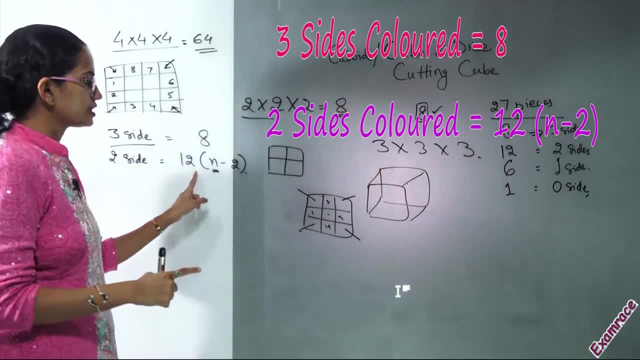 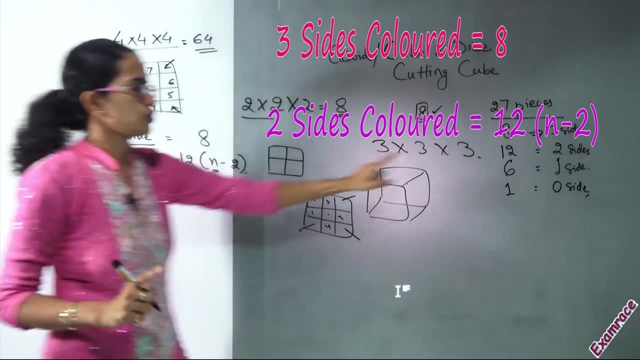 Here you are breaking it into 3. So you have 3 pieces. So let's try it for this case. So you have 3-2, that's 1.. 12x1 is 12.. So you have 12 pieces with two sides. 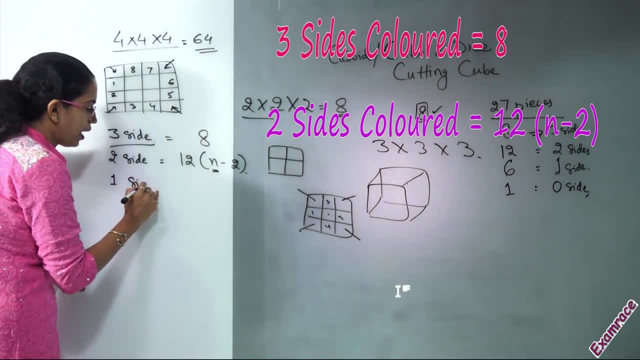 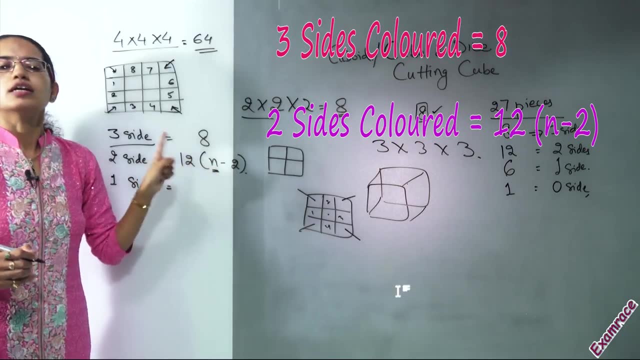 That makes it perfect answer. You have one side. Now, for one side, what would be the formula? You had no n that was here. You had one n that was here. In the next case, the value would go on to n square. 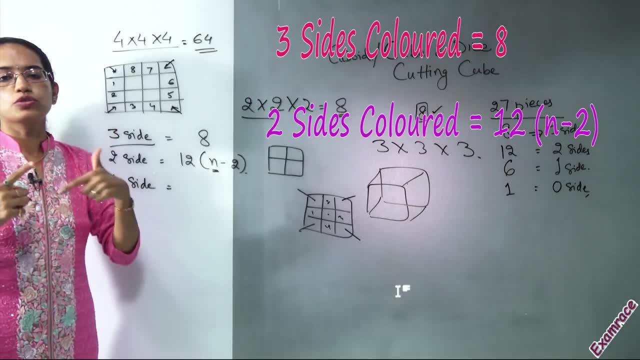 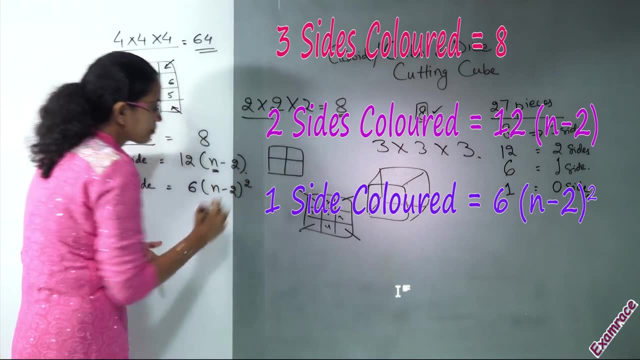 And in the zero side you would have value that would go on to n cube, And that's the way we remember it. So you have 6. n-2 square. So in this case it would be 3-2, that's 1.. 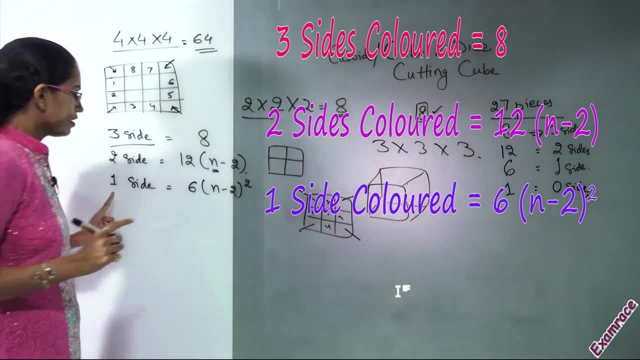 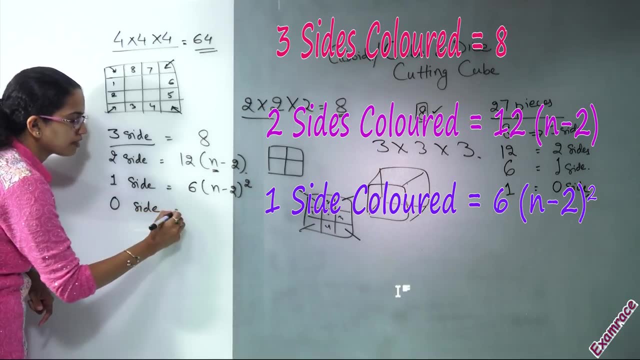 1 square, that's 1.. So it would be one side would be 6.. So 3x3, you have 6 as the correct answer And zero side. what would be the formula for zero side? For zero side, your simple formula would be: 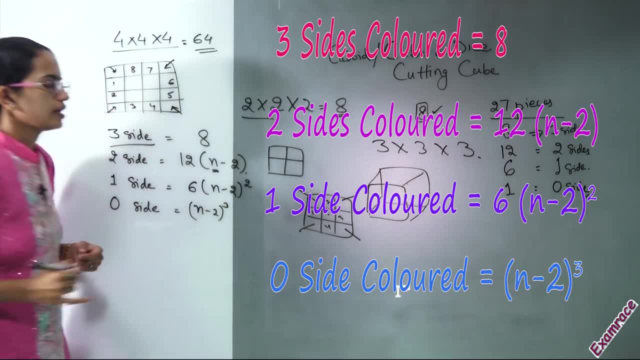 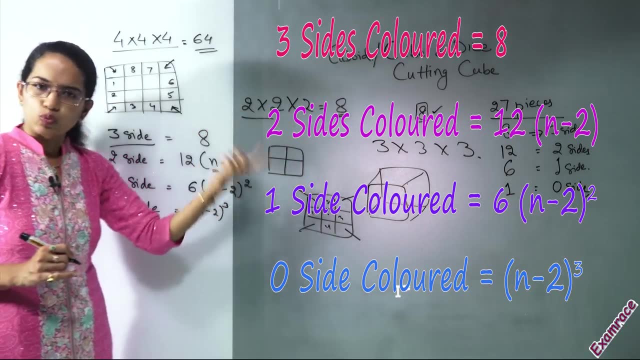 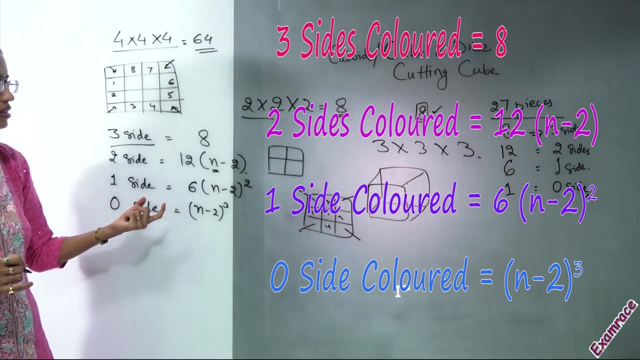 n-2 raised to power 3.. So in this case it would be 3-2, that's 1.. 1 raised to power 3, that's 1.. So you have sorry, that's 1.. 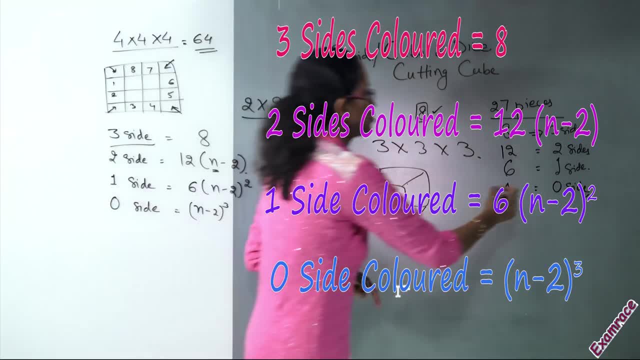 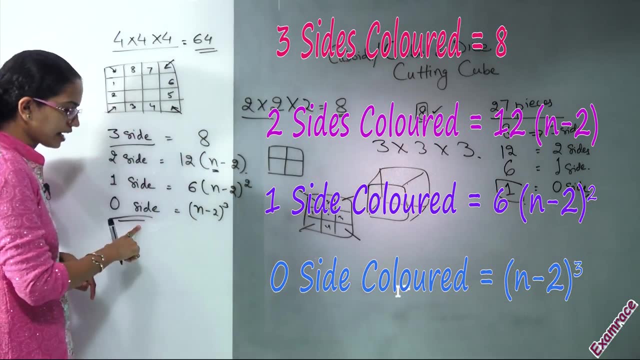 And you have 1 as the answer with zero side. So you have 1, that would be the answer for zero sides in case of 3x3.. And in case of 2x2, if we try to apply the same formula. 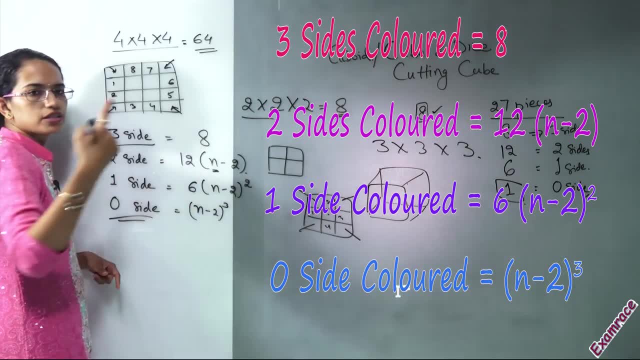 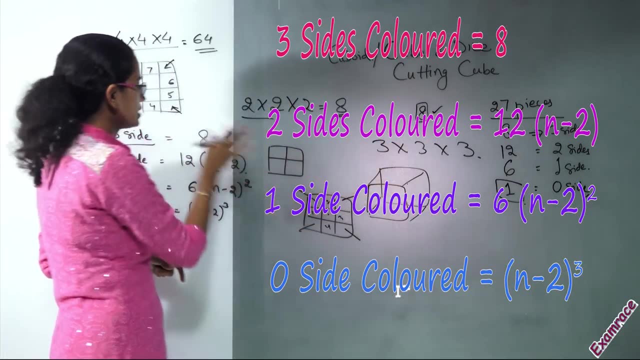 it would be 2-2, that's 0.. 0 raised to power 3 is 0.. So you would have 0 cube with zero sides. So that's how we understand the cube. Now, cube was pretty simple. You can remember the formula that we have for cube. 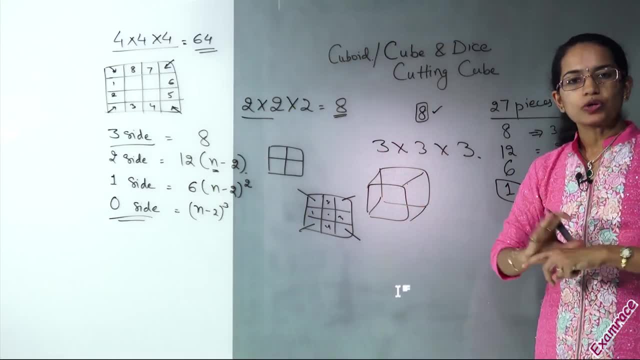 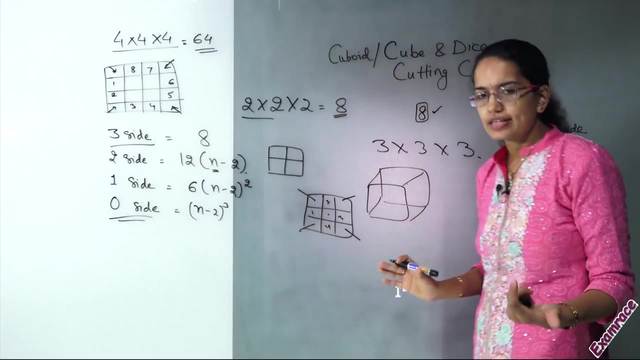 But in a while we'll proceed on to cuboid. So if you remember the formula for cuboid, you can automatically change it into cube. So you can do it either ways. So that's totally up to you. How do you proceed? 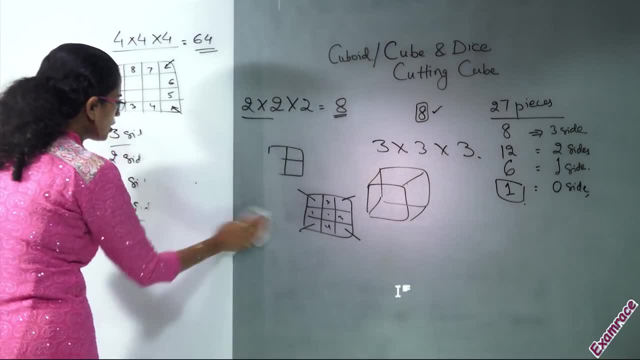 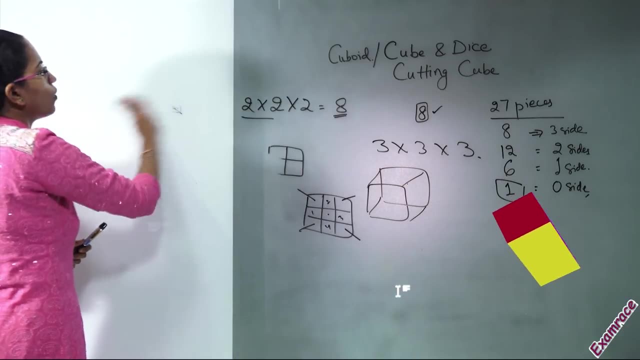 Now let's talk about cuboid. When we talk about cuboid, the only thing you need to remember here is: for cuboid, we can apply this formula only when we are able to cut the cuboid. In case you are not able to cut the cuboid, 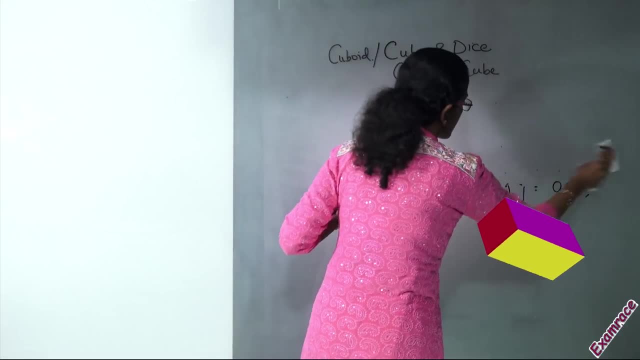 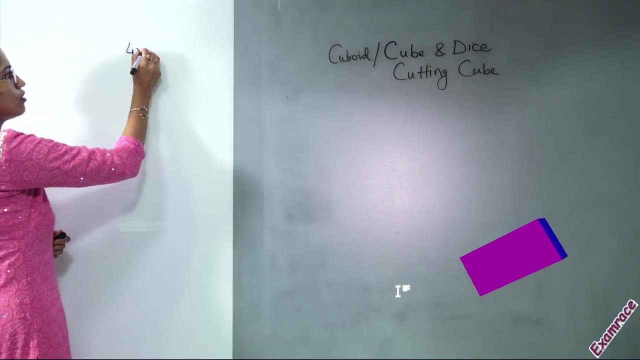 you cannot apply this formula. So that's a very, very fundamental and a very important concept that you need to understand. So, for cuboid, we will understand 3 cases: 4x2x1,, 4x2x2 and 4x2x3.. 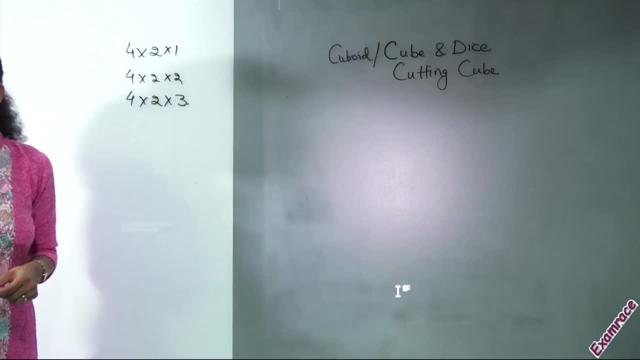 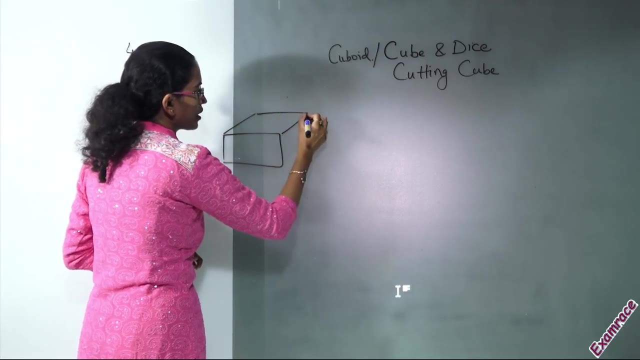 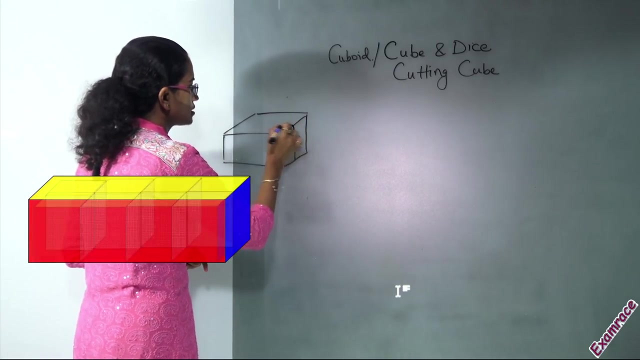 So those 3 cases we will understand. for cuboid Now the first cuboid that I am drawing is the first case. So let's say this is a cuboid. Now I have one side which has only one division. The other side has 2 divisions that are seen here. 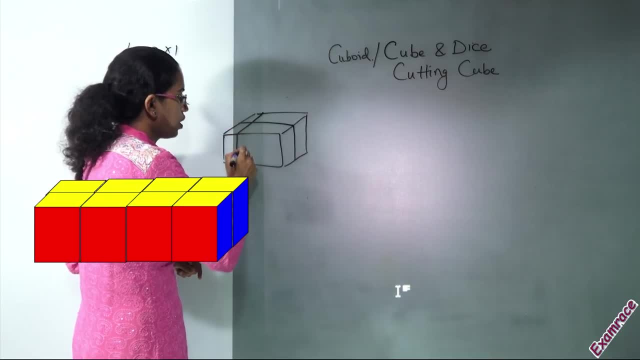 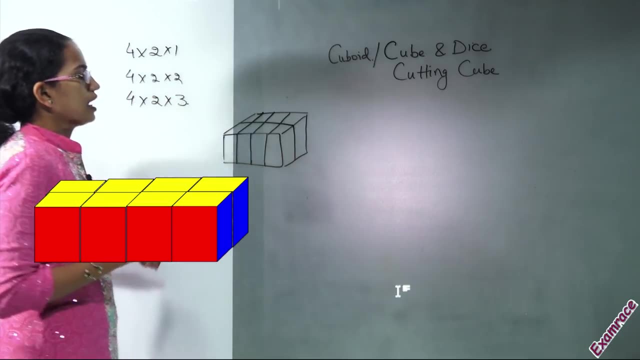 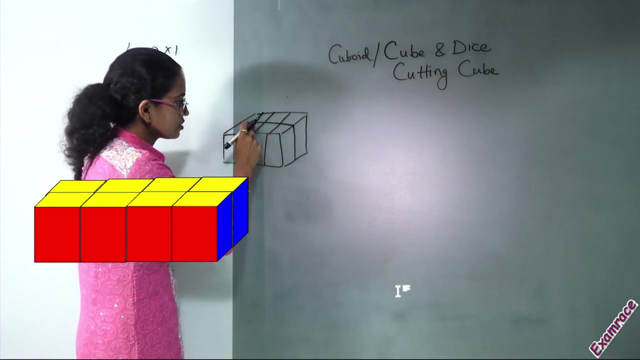 And the last side has 4 divisions. So I have 1,, 2,, 3 and 4.. Now, in this case, how many sides would be there which would have 3 colors? Now, in this case this, the center ones. 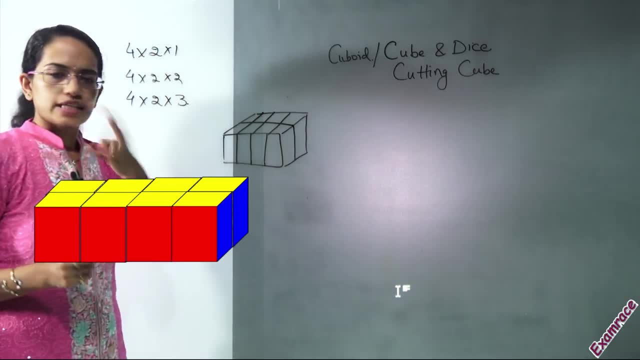 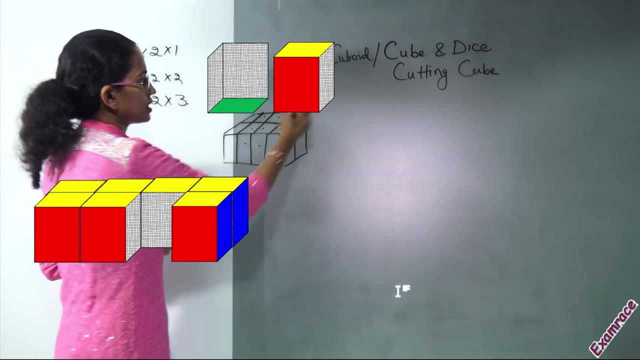 this one and these ones would have 3 sides- is colored because this side, this side and the bottom side, This side, this side and the bottom side, Similarly for this, this and the bottom side. So 4 pieces would be there which would have 3 sides colored. 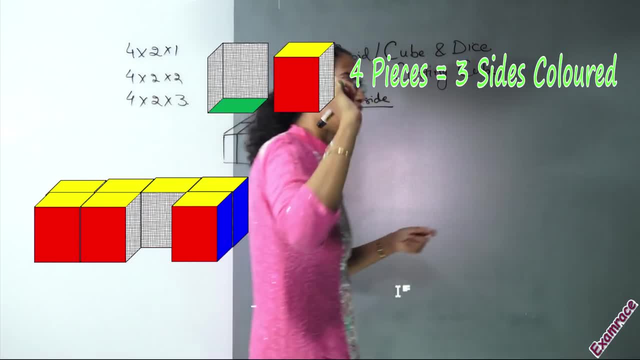 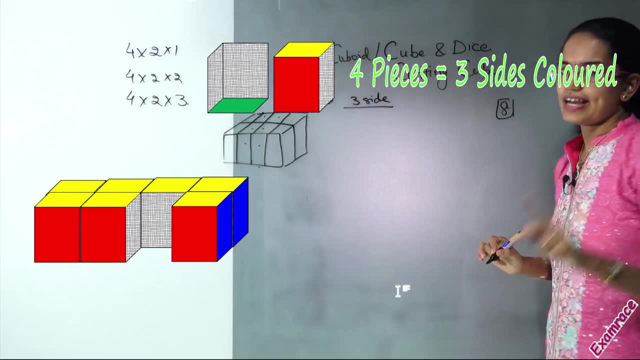 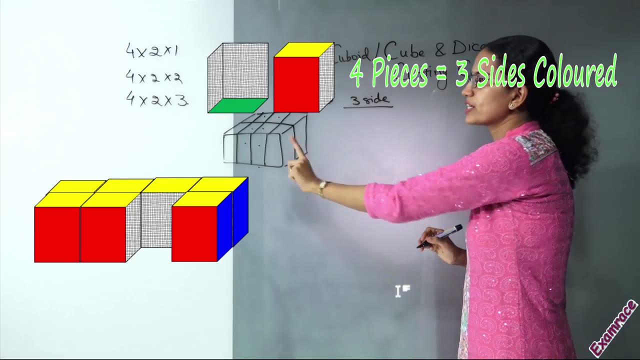 Now, so far, listen carefully, So far. in the case of cube, we were saying 3 sides. always you have 8 pieces. But, as I said, that applies only and only if you are able to cut it. In this case, you are not cutting it. 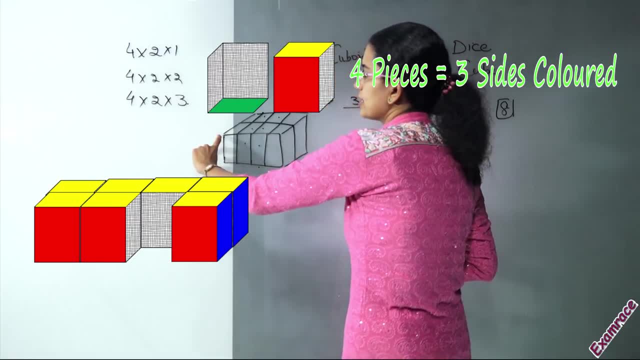 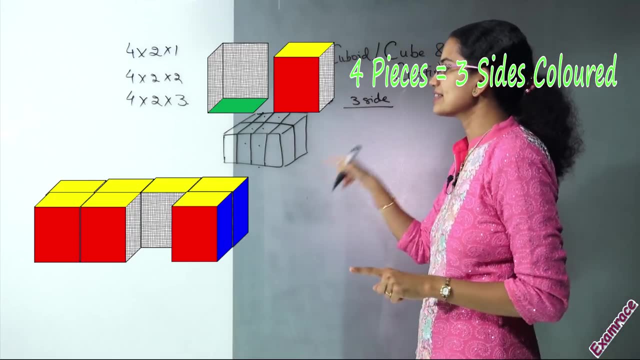 because one of the sides is just 1 cm And this 1 cm block I am leaving as it is. So you have 4 pieces which have 3 sides And in this case, interestingly, there would be 8 pieces which would have 4 sides as colored. 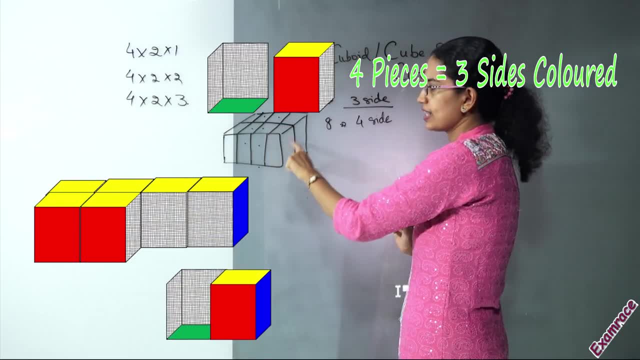 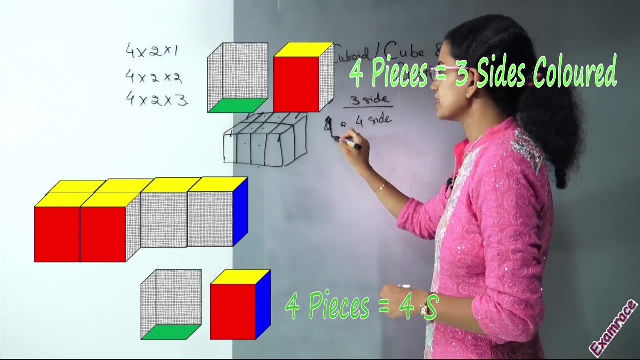 Now, this would be the top, the bottom, this side and this side, And similarly it would go for these, these, these and these pieces. So you would have 4 pieces, sorry, 4 pieces, which would have 4 sides as colored. 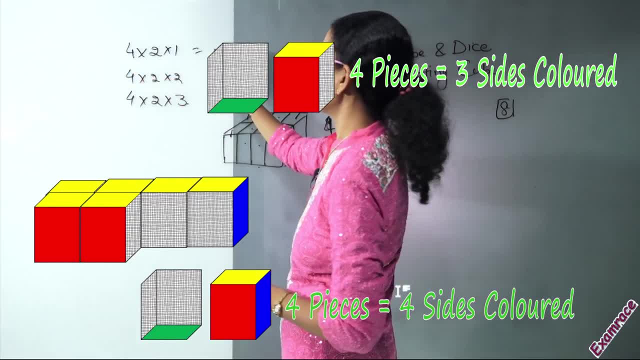 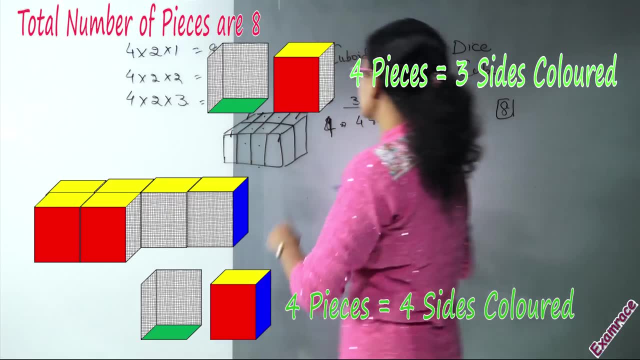 And how many total pieces would be there. It is 4 x 2 x 1,, that's 8 pieces. In this case, you would have 16 pieces And in this case you would have 24 pieces. So in this case you would have 4 pieces with 3 sides colored. 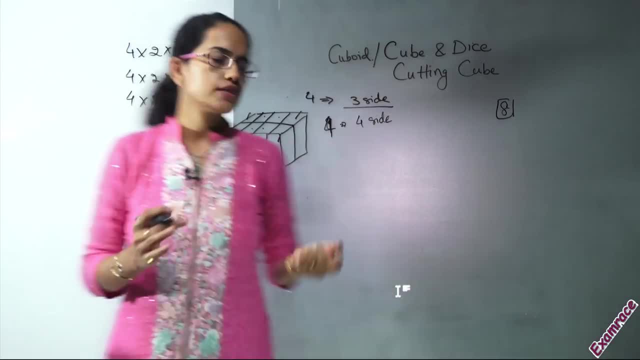 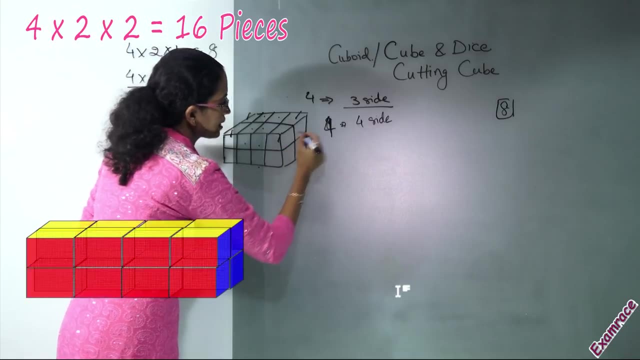 and 4 pieces with 4 sides colored. Now what I do is the same diagram. I do it 4 x 2 x 2.. So what I do is I create an extra line here So it becomes 2 x 2 on 2 sides. 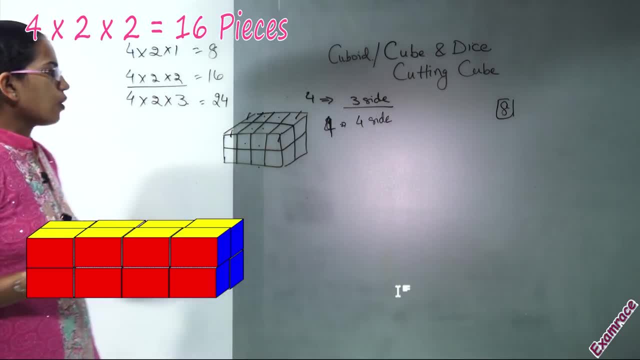 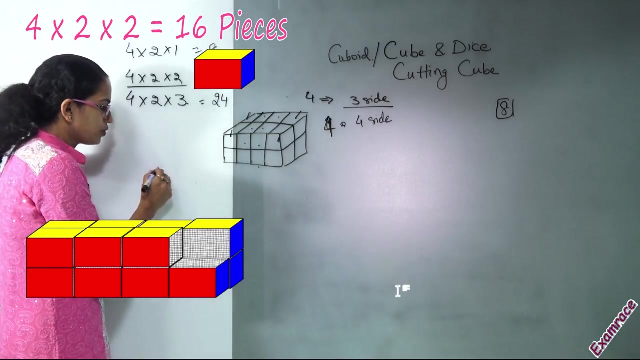 and 4 x 2 on 1 side. Now, in this case, what you can visualize is- it's again pretty simple. So in this case you can understand how many pieces would be there which have 3 sides colored. So you would have 8 pieces. 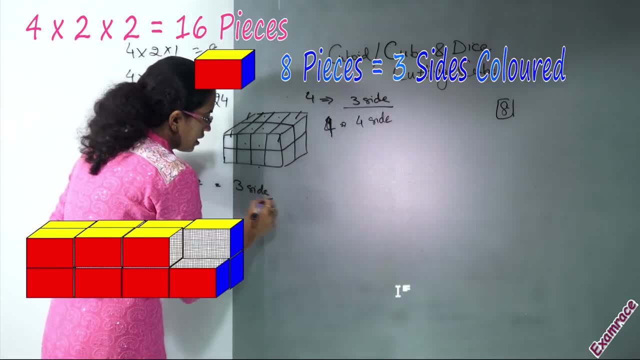 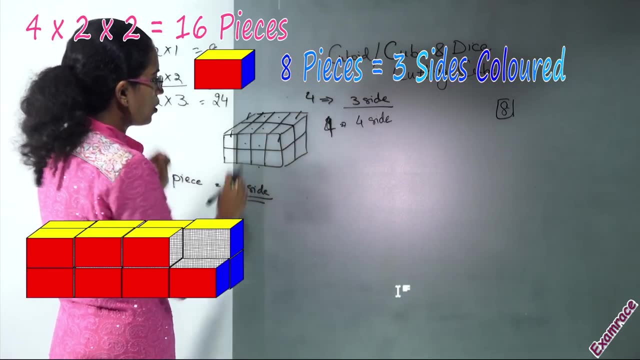 which would have 3 sides colored In all. how many pieces are there In all? only 16 pieces are there. Now the corner pieces that are there are gone. How many pieces are there with 2 sides colored? So you have the middle 8 pieces. 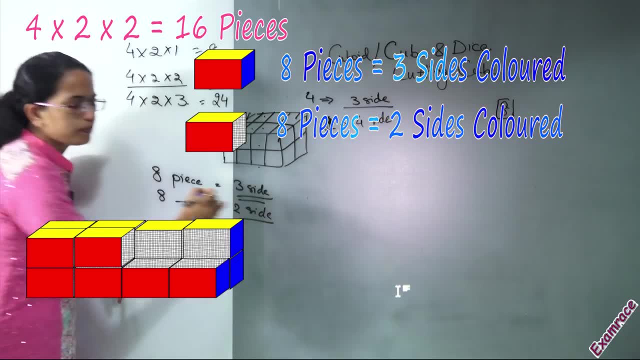 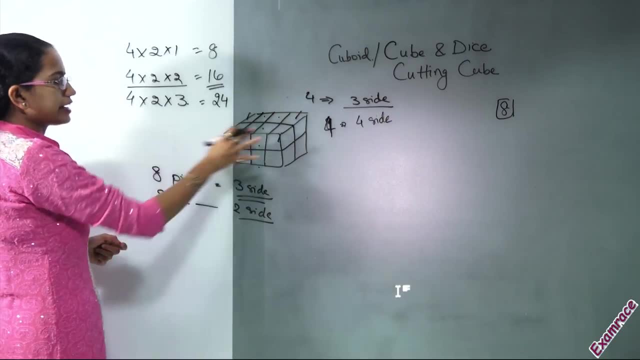 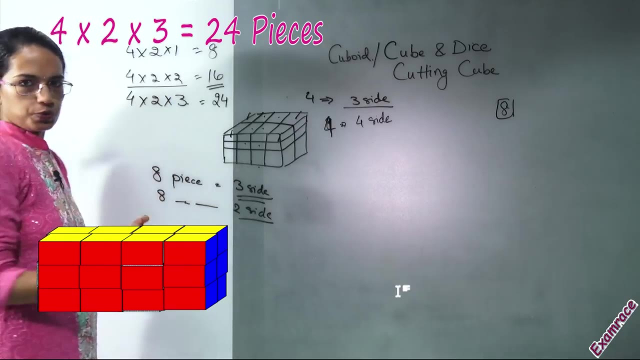 with 2 sides colored, So there are no pieces which have 1 side or 0 side colored. in this case, Again, what I do is I take the same cube, I draw one more line And this makes it 4 x 3 x 2.. 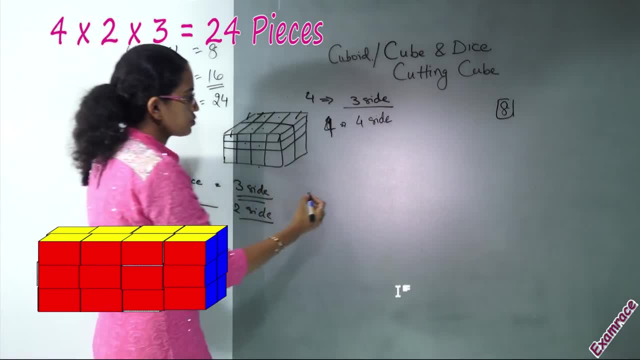 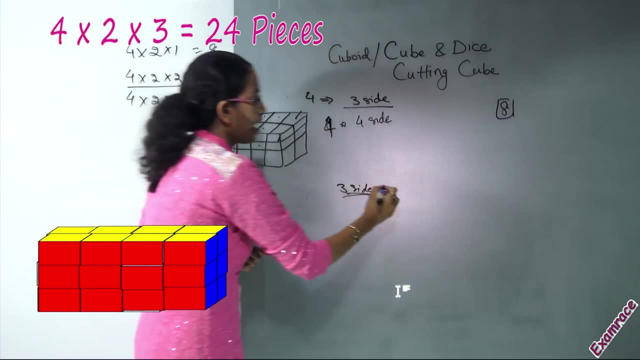 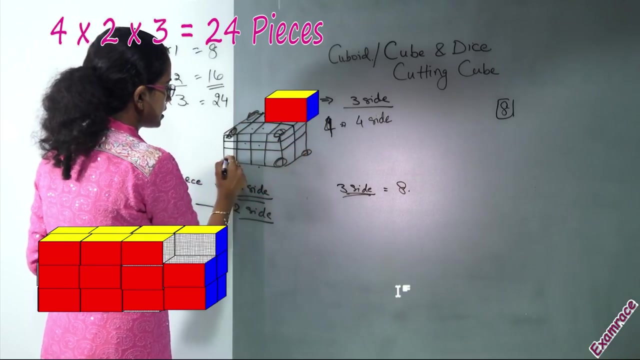 Now, in this case, how many pieces would be there which would have 3 sides colored? So 3 sides. when you are able to cut the cube at least once, you would have 8.. So you can see 1,, 2,, 3,, 4,, 5,, 6, 7. 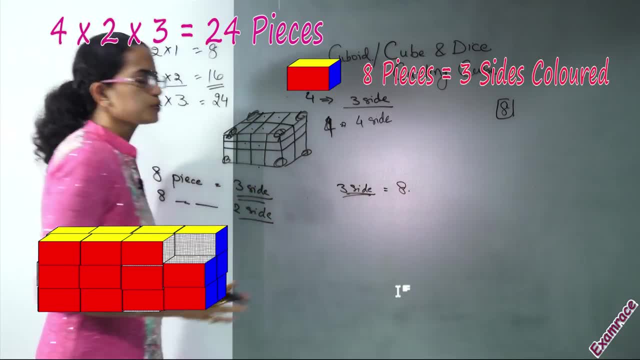 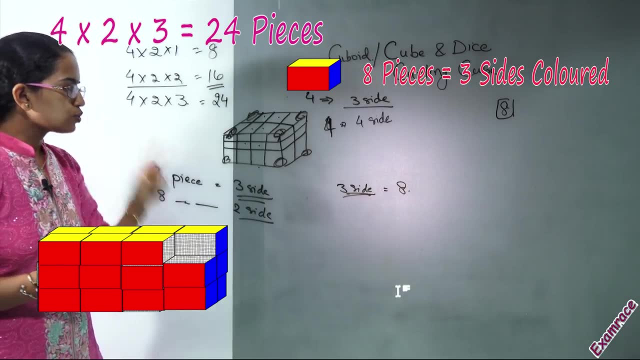 and 1 on the back side, so 8.. So 8 cubes would be there which would have 3 sides colored. How many cubes would be there which would have 2 sides colored? So, for 2 sides colored, how would you calculate? 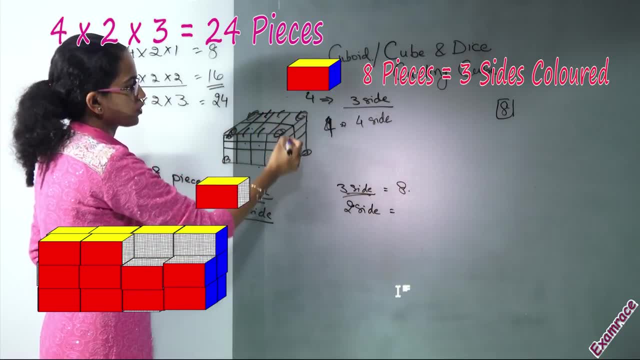 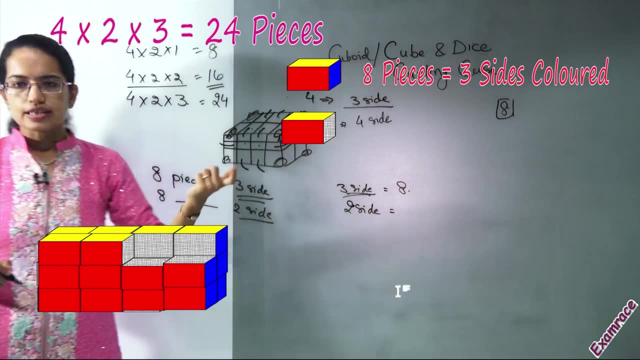 You would have 1 cube, 2 cube, 3 cube, 4 cube, 5 cube, 6 cube, 7 cube, 8 cube, 9 cube, And then on the other side you would have 10 cube, 11 cube. 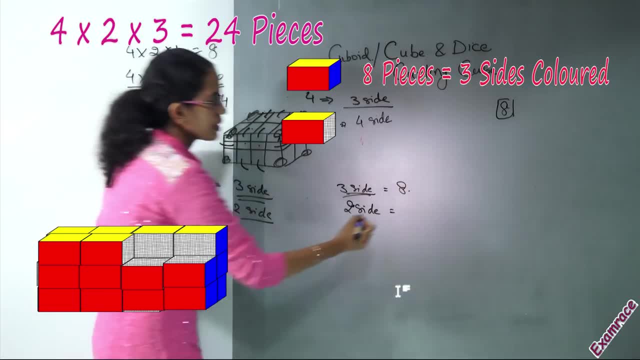 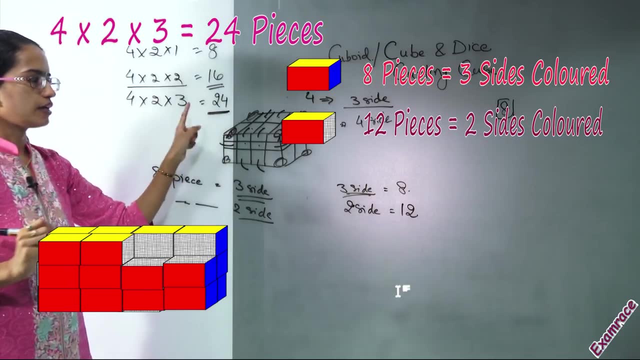 and 1 on that side, So 12 cubes. So there would be 12 cubes which would have 2 sides colored. And how many are total? There are total 24.. We already have 20 cubes that are done. Now how many cubes would be there? 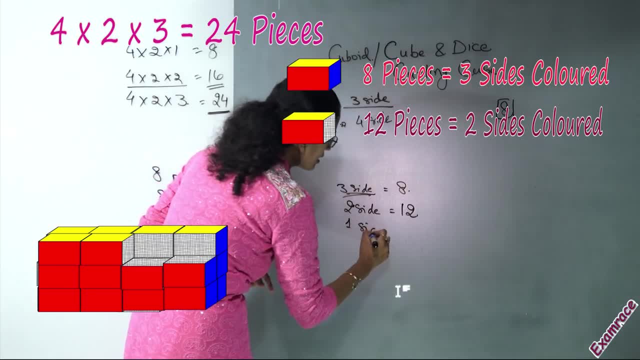 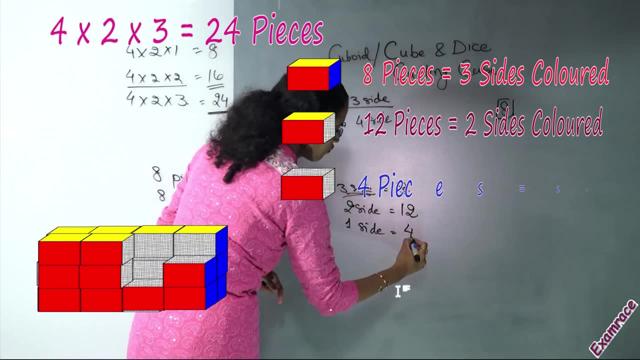 that would have 1 side colored. So 1 side colored, how many cubes would be there? 2 on this side and 2 on the opposite face of this. So it would make it 4.. And therefore you have 24 cubes. 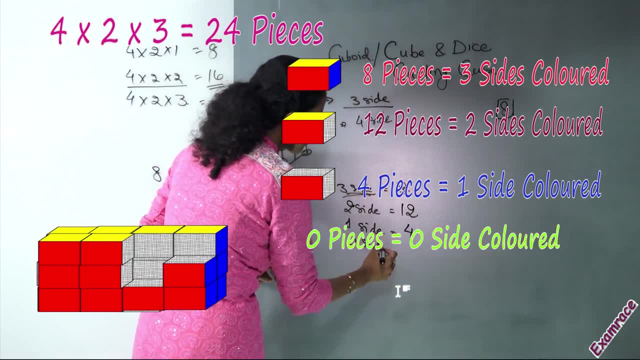 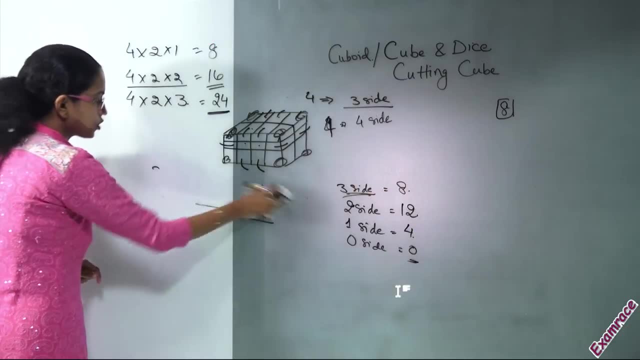 You do not have any cube which has 0 side. So 0 cubes with 0 side. So that's how we find it for a cube, sorry cuboid. Now, when you are cutting a cuboid into smaller cubes, indeed, Now, what are the formula? 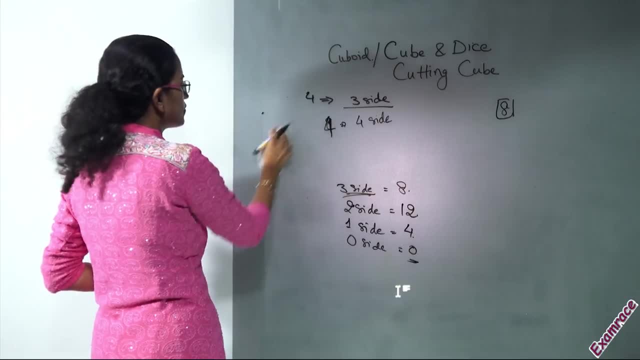 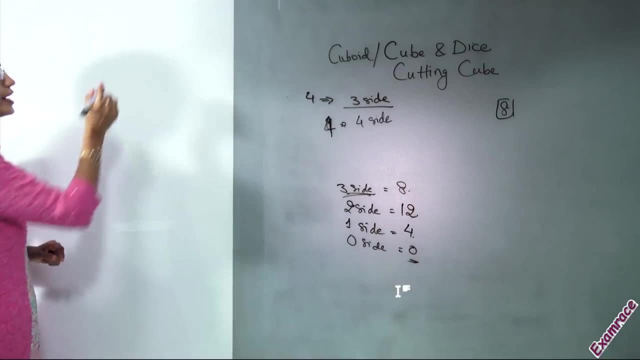 that we use for cuboid. Let's understand this and then we will translate the same formulas to cube and see how you can remember those. So for cuboid, you have 3 sides which are painted, You have 8. That's similar to what we saw. 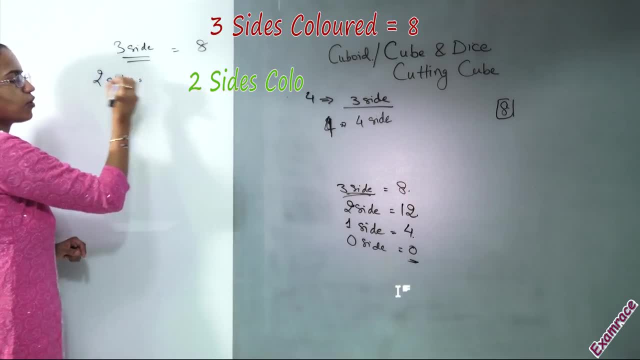 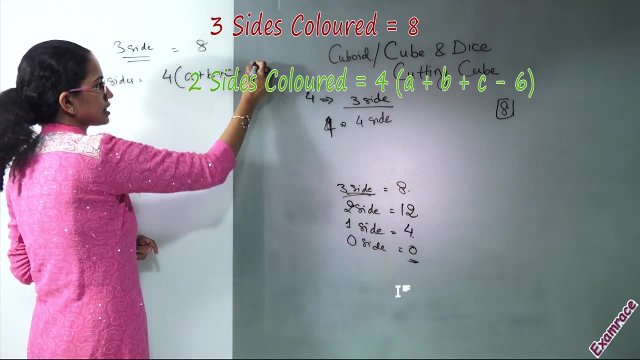 in the case of cube, For 2 sides. what is the formula For 2 sides? your formula is simple. It's 4 into a plus b, plus c minus 6.. Okay, Then, what is your formula for 1 side colored? 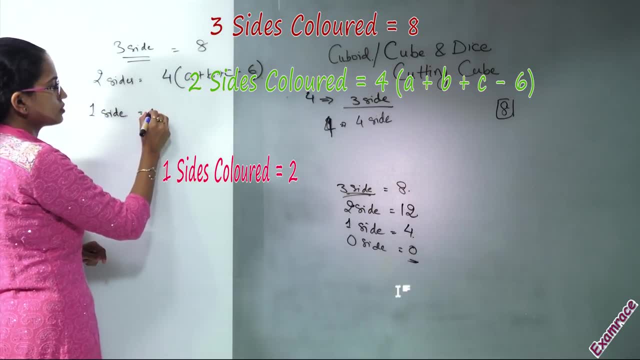 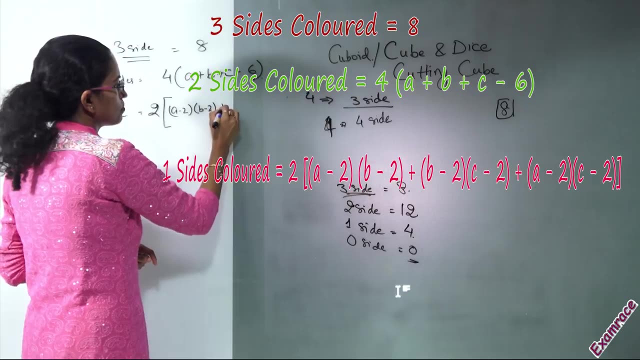 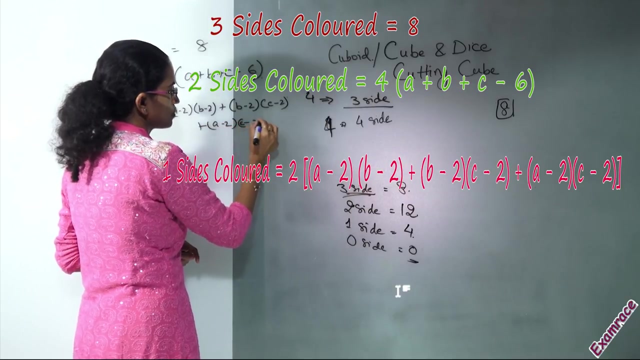 So for 1 side colored, your formula comes out to be: it comes out to be: 2: a minus 2, b minus 2 plus b minus 2, c minus 2 plus a minus 2 and c minus 2.. So that's the formula for. 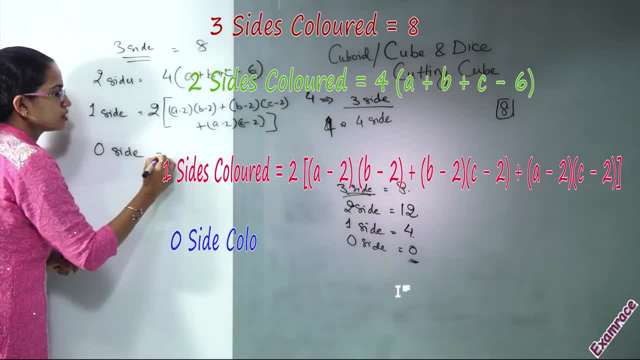 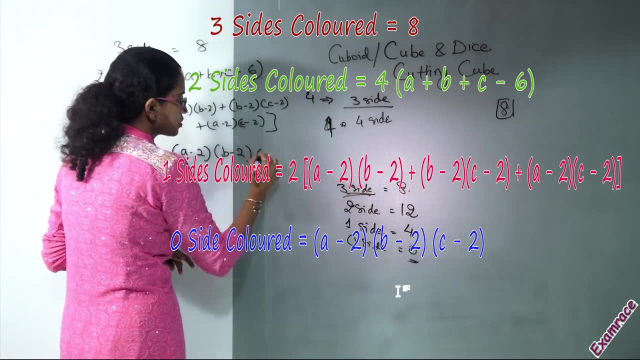 1 side colored. And what's the formula for 0 side colored? For your 0 side colored, the formula would be a minus 2 into b minus 2 into c minus 2.. Now these a, b, c are the. 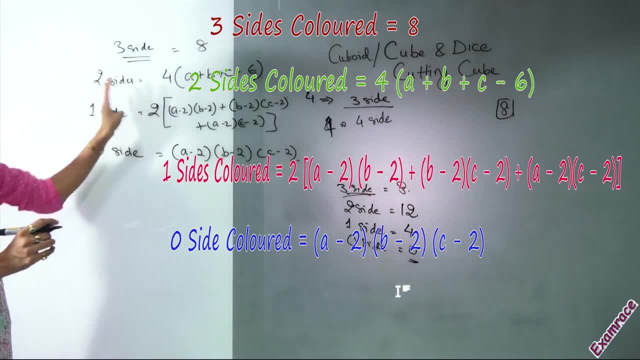 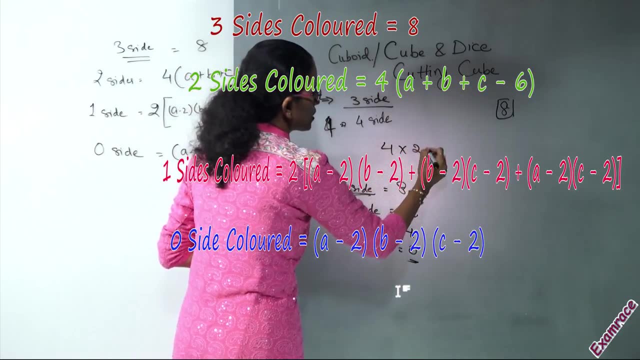 3 different sides. Now let's apply this formula. This formula, as you cannot see, as you can see, cannot be applied for the first case where we took 4 into 2, into 1. Because, since it's 1, you would have a negative values. 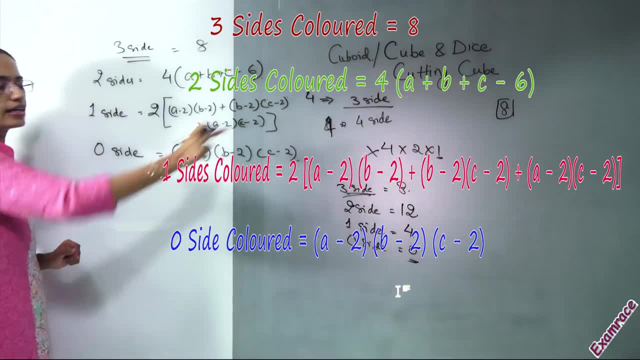 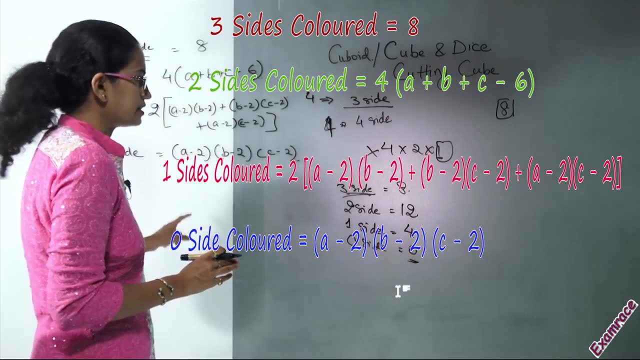 that would be there, and this formula cannot be applied until and unless you are cutting a cube. So since one of the dimensions is 1 and this dimension is not being cut, you cannot apply this formula. You can apply this formula only when you are cutting. 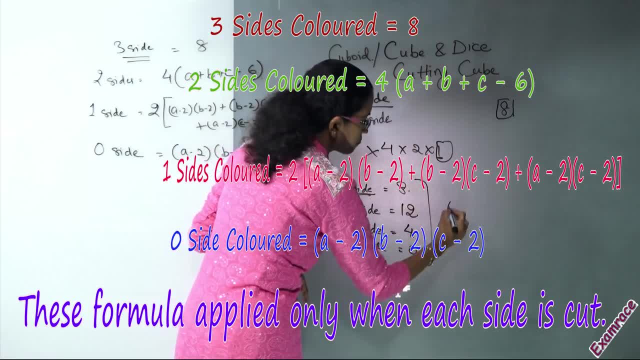 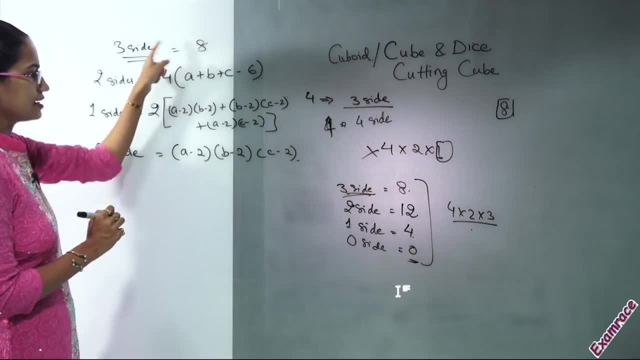 the dimensions. So this was the case that we derived for 4 into 2, into 3.. Now, applying this here, let's talk about one side. that's the critical. The others you can directly find out. So for this you would add it as: 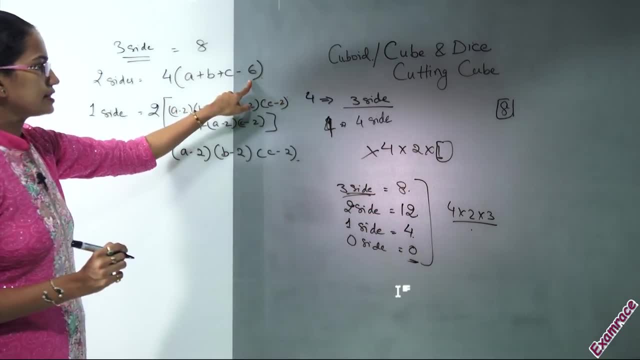 4 plus 2 plus 3, that makes it 9.. 9 minus 6 would be 3.. 3 into 4 would be 12.. So you have 12 as your answer, But when it comes to one side, 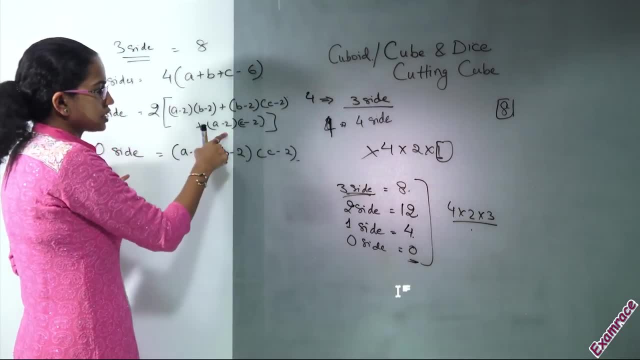 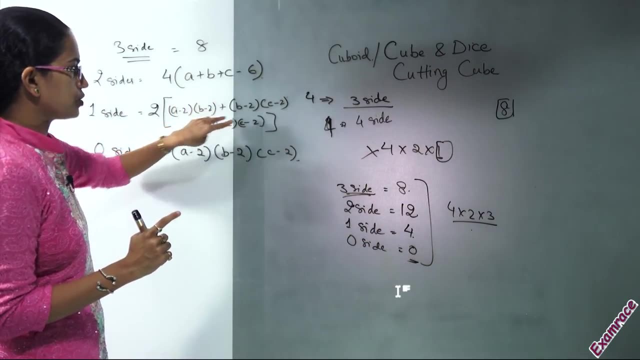 what would happen In two cases. you are using a minus 2.. So wherever you are using 2 minus 2, it would be 0. So two of the values would go on to be 0. And one of the values would be 3 minus 1.